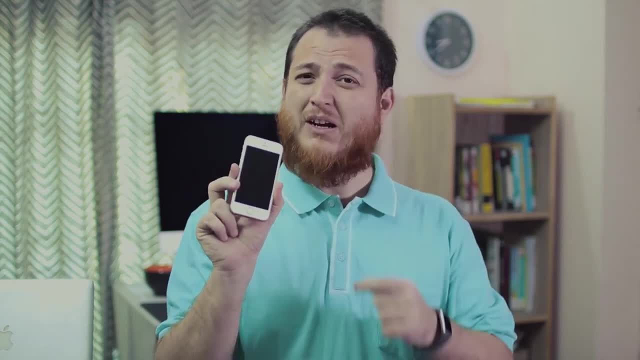 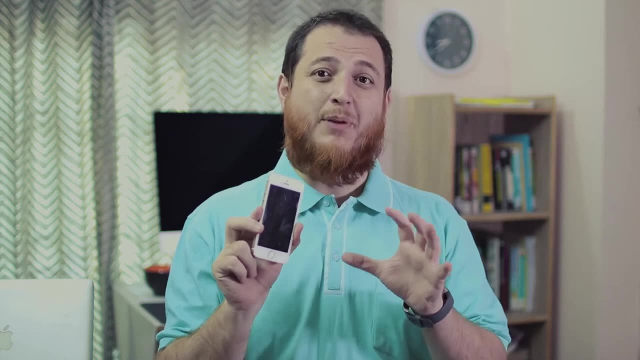 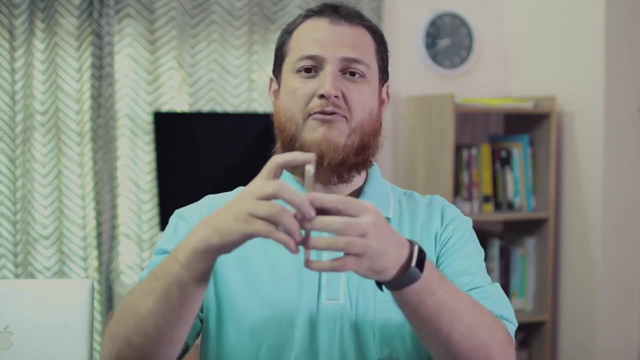 dark so I need to turn it off. But where I am going to turn it on or which button I am going to press is going to be signified by using signifier. So I am going to show you the buttons over here. So here we have one button at the top and if you see it closely, then we have three buttons. 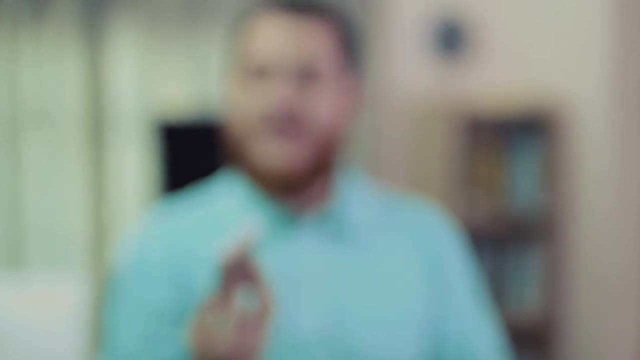 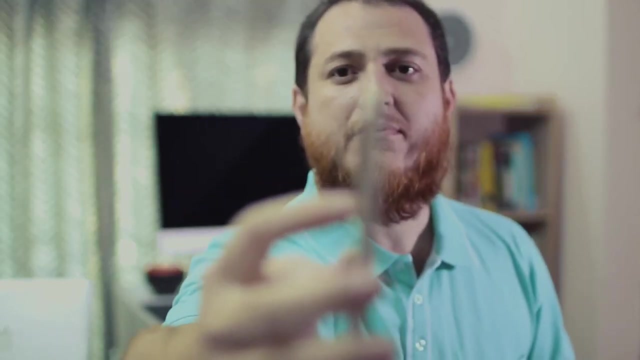 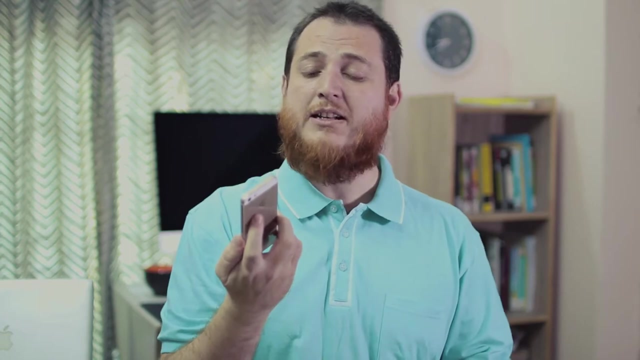 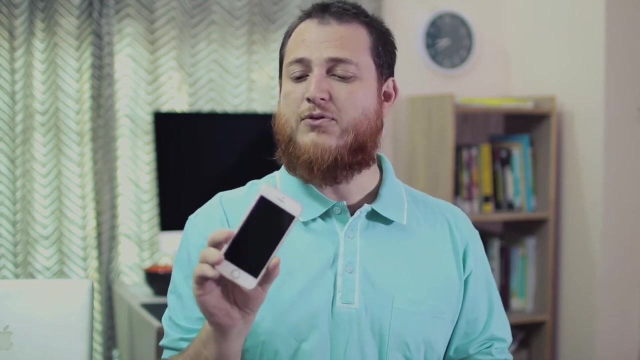 on this side. You can see over here and you can see that they have plus. Let me show you, Let us zoom in. Okay, so it's not zooming in, but there is a plus symbol on one button and minus symbol, which signifies that it is going to increase or decrease the volume of this mobile phone. 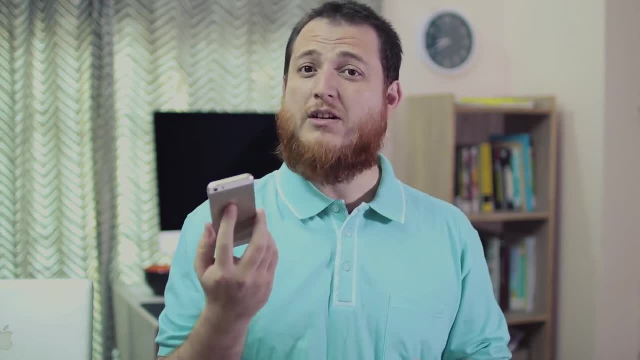 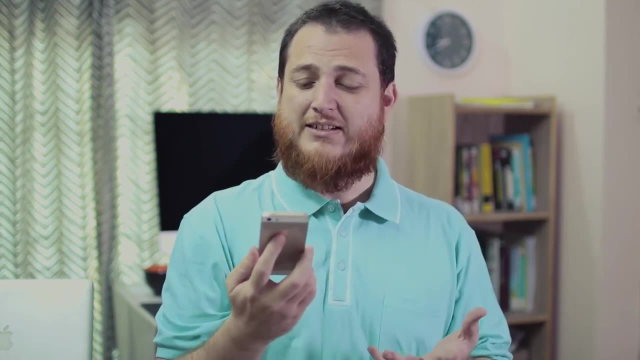 And the mute button. for the first time, I didn't know what is going to do this button, Whether it is going to mute or it is going to dim my screen colors or whatever. But after using it once, I knew that this is going to mute it. 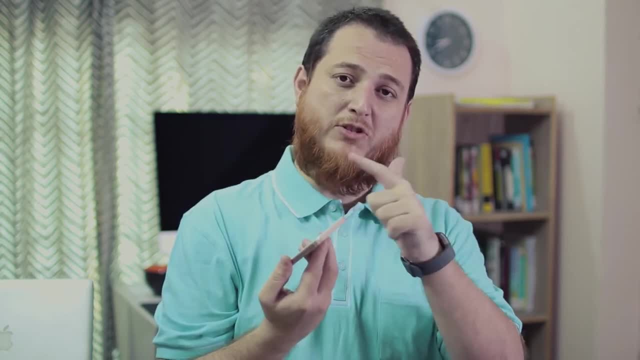 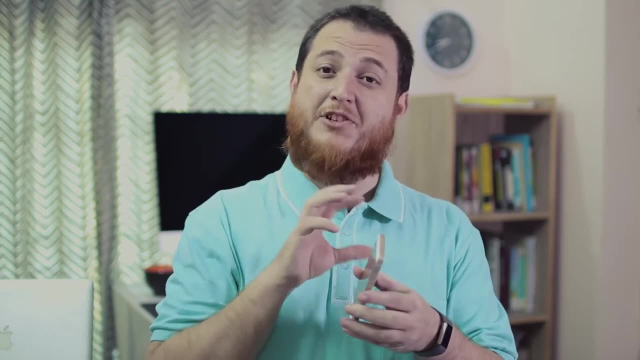 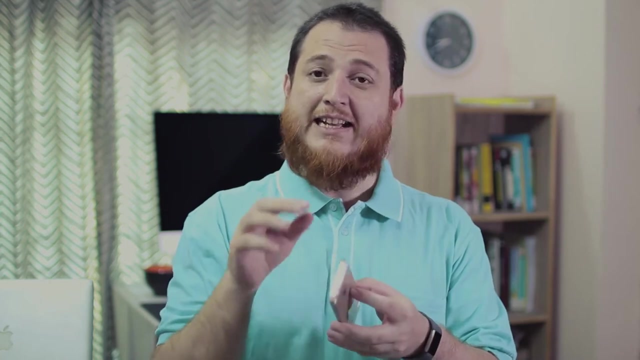 If they had put some icon over here that it is going to mute, then that would be more helpful. Okay, so always there will be some trade-off between design and signifiers. You can see over here that they can put. they can make this button, this turn on button at the top you can see over. 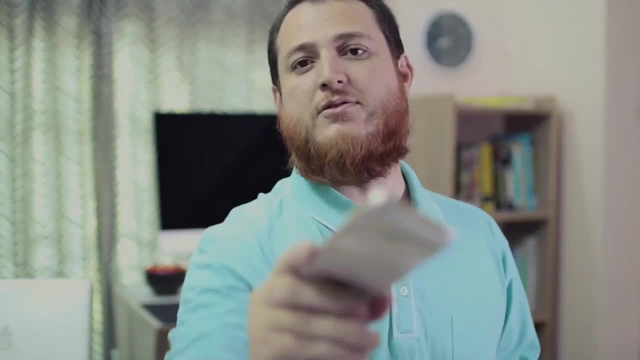 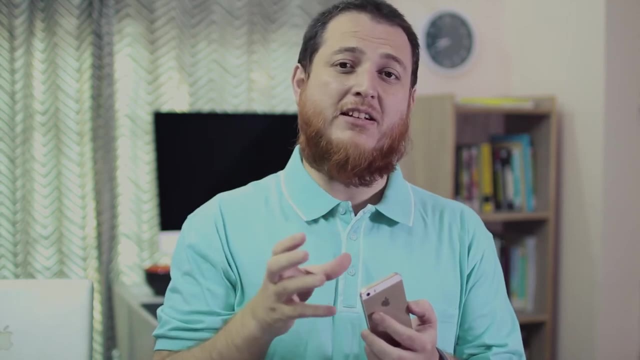 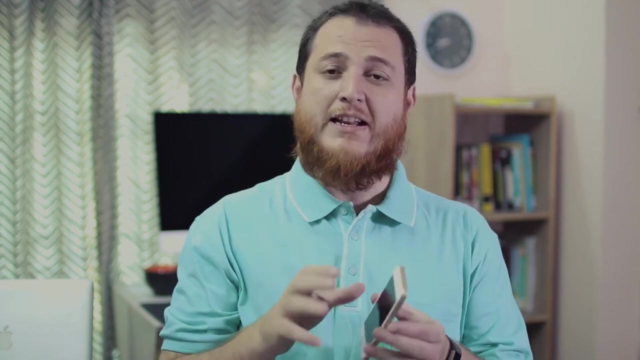 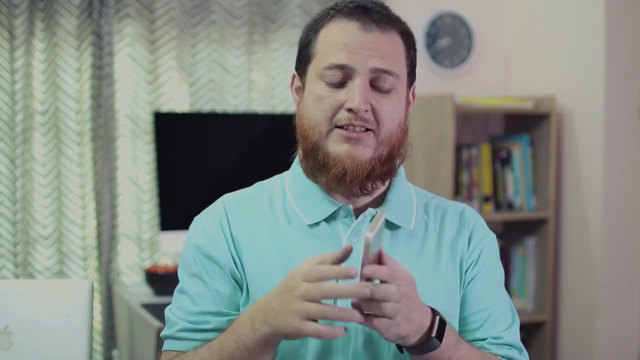 here. Okay, so this is not focusing anyhow. Okay, the button at the top if it's a bit different color, like red or maybe green, so I know that I am going to press this to turn it on. Right now, when I use this for the first time, I'm not going to be sure which button is going to turn on this device. 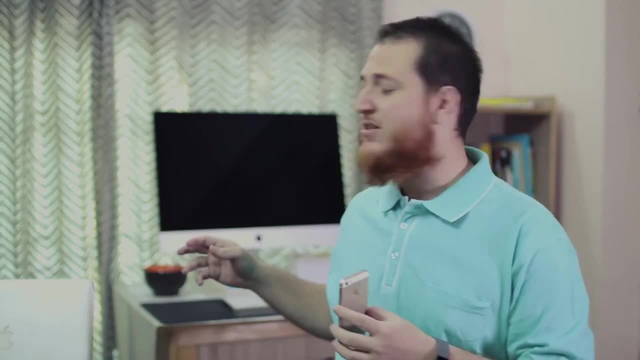 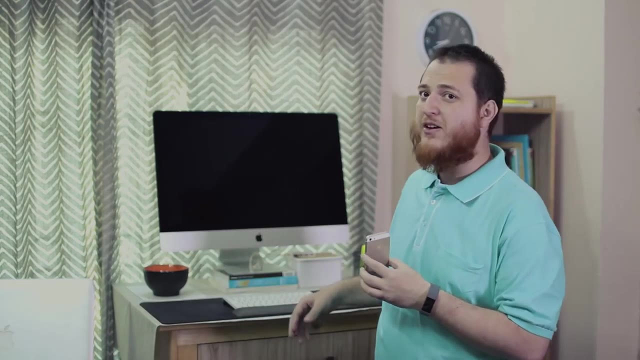 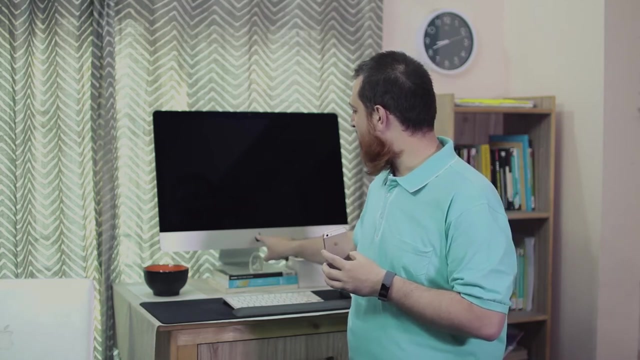 Similarly, if you see my iMac at the back, you can see over here. this is my iMac. and when I first showed my iMac to one of my friends, you can see that there is an Apple logo over here. and what he did is he tried to tap over here like.